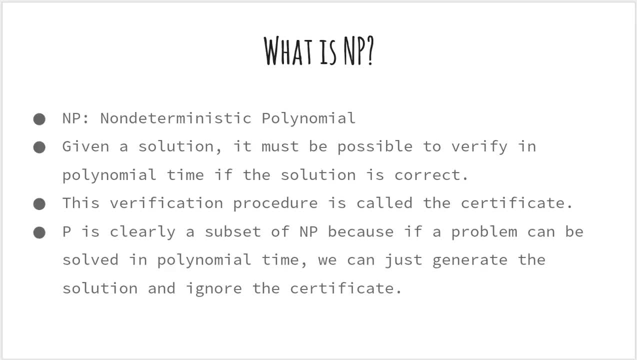 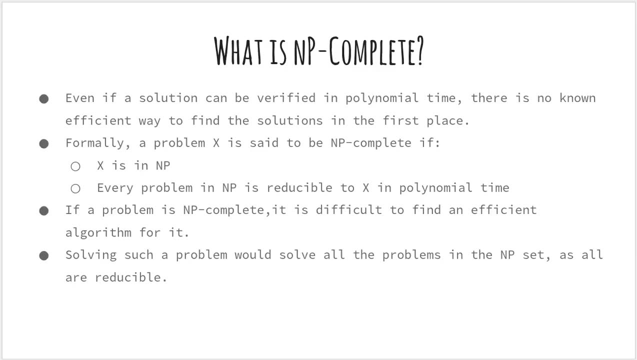 we can just generate the solution in NP. We can ignore the certificate. Now we will talk about what NP complete is. We believe that some problems are intrinsically unsolvable by polynomial time algorithms, Although the solutions can be verified in polynomial time. 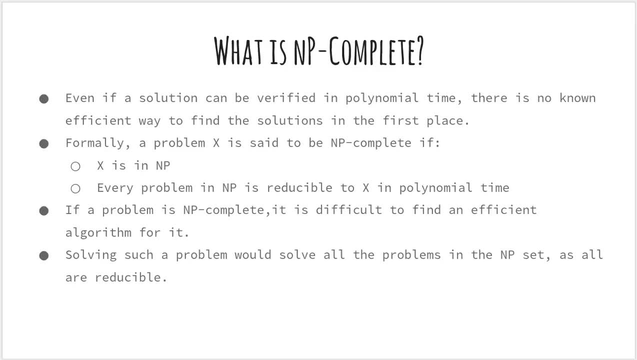 there is no known efficient way to find these solutions in the first place. Formally, a problem X is said to be NP complete if X is in NP and every problem in NP is reducible to X in polynomial time. From a practical point of view, 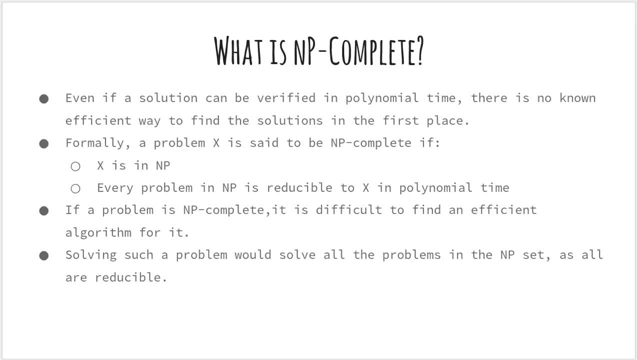 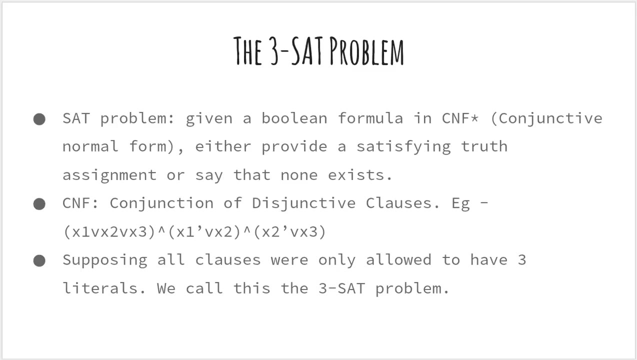 discovering a problem is NP complete indicates that you will have difficulty finding an efficient algorithm for it. If you could, you would also have solved every known NP complete problem, as all these problems are polynomially reducible to each other. Let's examine one of these problems. 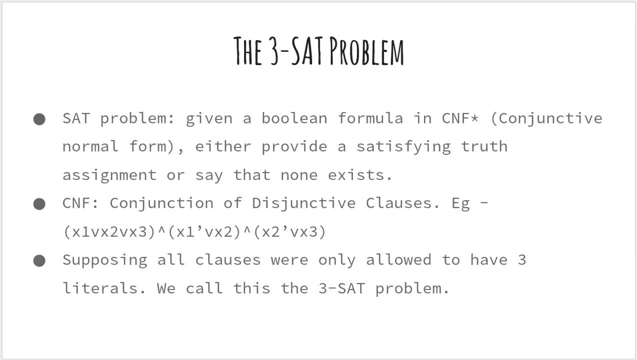 It's called the 3SAT problem. Okay, we will start off with the SAT problem. What is a SAT problem? That's supposing you are given a Boolean formula in conjunctive normal form. You must either provide a satisfying truth assignment or say that none exists. 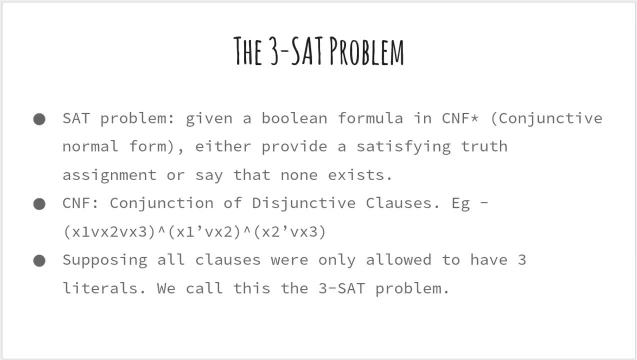 What is conjunctive normal form? It's nothing but a conjunction of disjunctive clauses. So disjunction is nothing but the OR operator. So what you are essentially saying is that you have a Boolean formula that is made up of clauses. 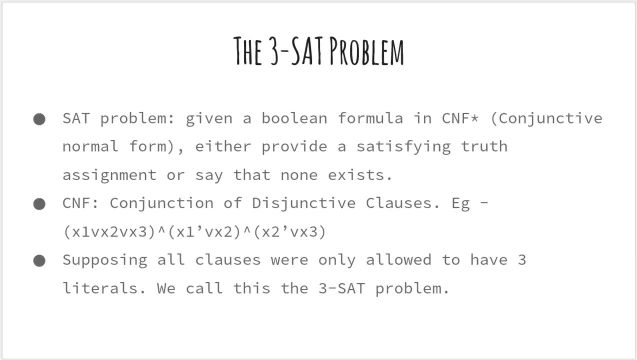 These clauses are ANDed or are in conjunction. Within these clauses, all the literals are ORed or are in disjunction. Now suppose that each of these clauses was only allowed to have three literals, at most three literals. We call this the 3SAT problem. 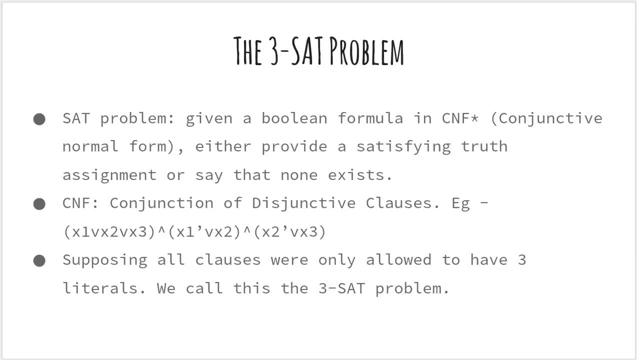 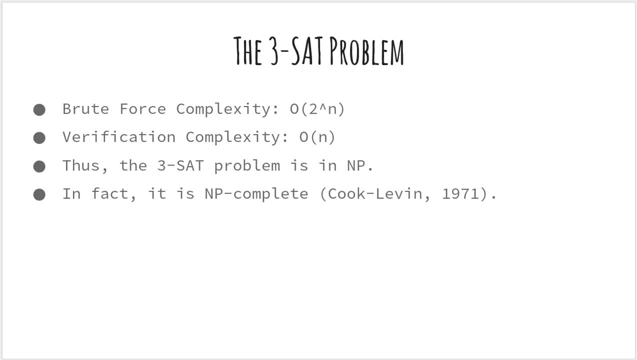 The 3SAT problem is nothing but a special case of the SAT problem. Okay, so we have the 3SAT problem. So one way of solving the 3SAT problem is you can try every possible combination of truth assignments for the n variables. 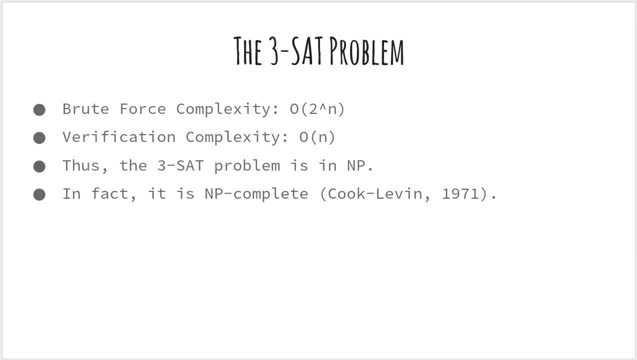 So it's clear to see that there are 2n such possibilities. So if we tried this approach we would be running in O. But if somebody gave us the solution then it's very easy to see that if it satisfies the Boolean formula. 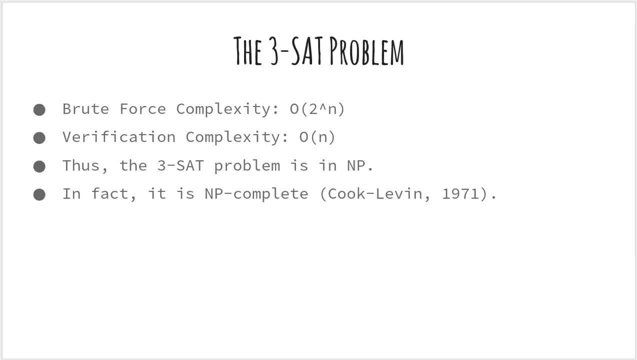 So these are the two conditions for NP right, That even if the problem itself is not solvable, if someone generated a solution, you should have a certificate that runs in polynomial time that says whether the solution is valid or not. So thus the 3SAT problem is in NP. 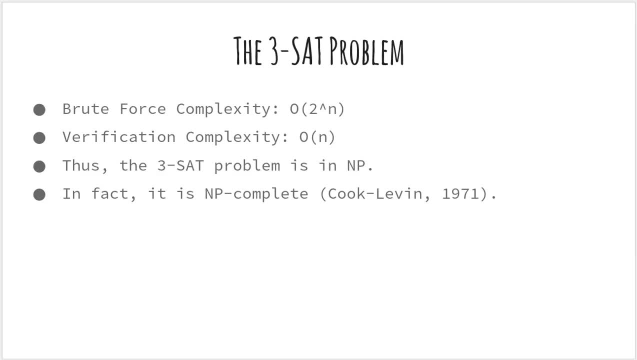 In fact it is NP complete. It was one of the first known NP complete problems and it was independently solved by Cook and Levin in 1971 and 1973. And this problem is often used as a starting point to show that other problems are NP complete. 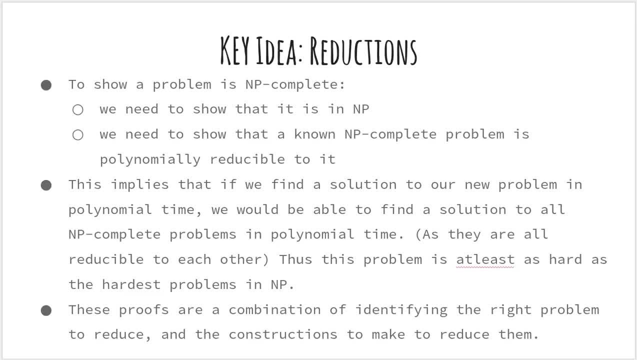 So this brings us to an interesting junction. To show that a problem is NP complete, we need to show two things: One, that it is in NP and second, that we need to show that a known NP complete problem is polynomially reducible to it. 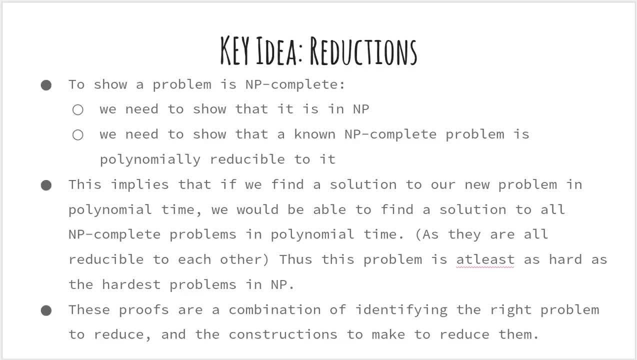 So this implies that if we found a solution to a new problem in polynomial time, we will be able to find a solution to all NP complete problems in polynomial time, as they are all polynomially reducible to each other. Thus this new problem is at least as hard as the hardest problems in NP. 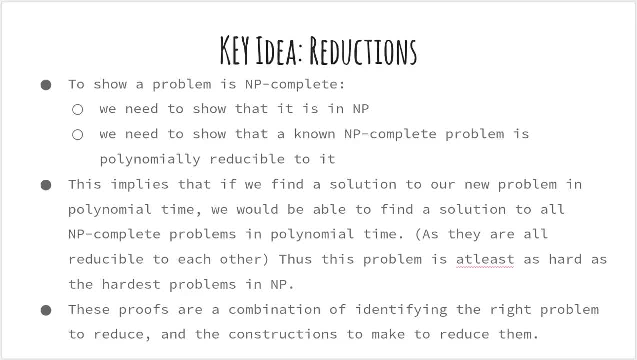 So all these proofs are a combination of identifying the right problem to reduce and the constructions to make to reduce them. Why do we choose only one problem to reduce? Because if we are able to prove that one problem is reducible to our problem, 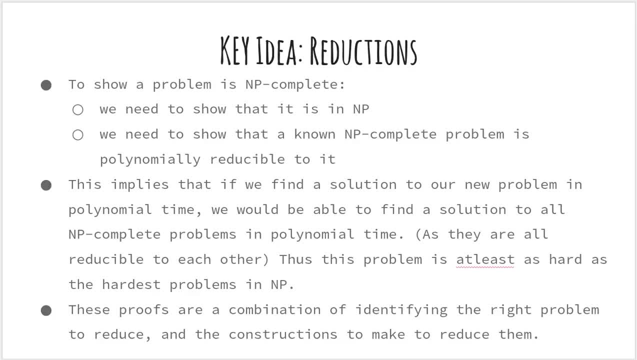 then every other problem in the class of NP complete is reducible to that problem in polynomial time. So by extension, we have shown that our problem is at least as hard as any of the NP complete problems. Alright, now we will look at a few interesting problems to elucidate this idea further. 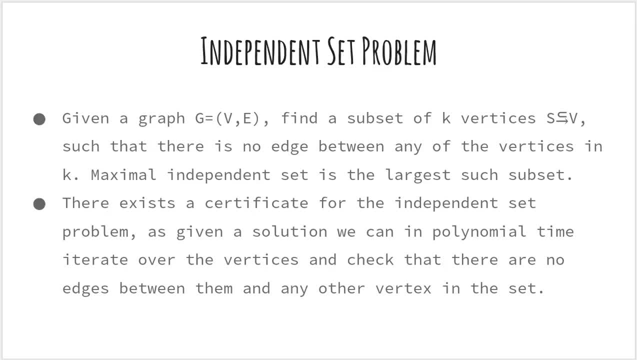 So the first such problem we will look at is the independent set problem, which asks that, given a graph G, can you find a subset of k vertices such that there is no edge between any of the vertices in k? The maximal independent set problem is the question of finding the largest such subset. 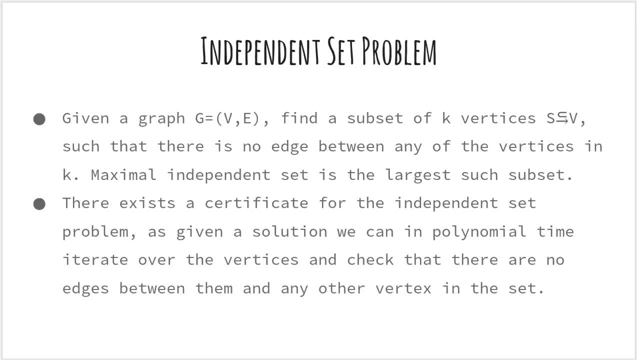 So there exists a certificate for the independent set problem. certainly, As someone gave you the k vertices in a graph G, you can easily iterate over the vertices and check that none of them have an edge to any other vertex in that subset. So this shows that the independent set problem is in NP. 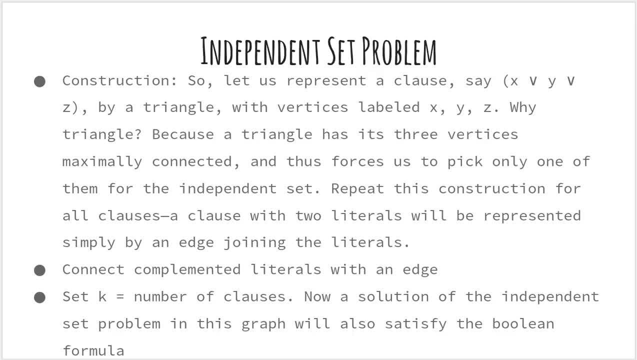 Now we need to show that the independent set problem is NP complete. To do this, our first step is to pick a problem to reduce to the independent set problem. We have just seen the 3 set problem, so we will choose that problem to reduce to the independent set. 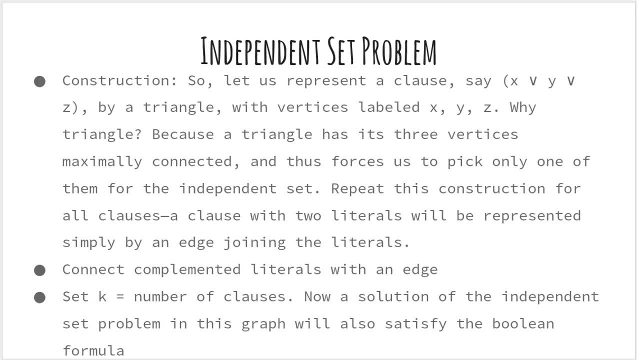 So, supposing you have a clause in the 3 set problem, say it's x or y or z, You can represent this clause by a triangle, with each vertex labelled x, y, z. Now construct a graph G where each of these clauses are represented by a triangle. 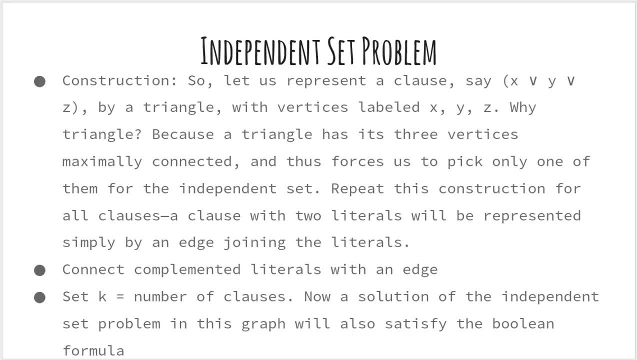 Draw an edge between each literal and its complement. Why do we choose triangles? Because a triangle has its 3 vertices maximally connected and thus forces us to pick only one of them for the independent set. because if you pick 2 of the vertices of the triangle, 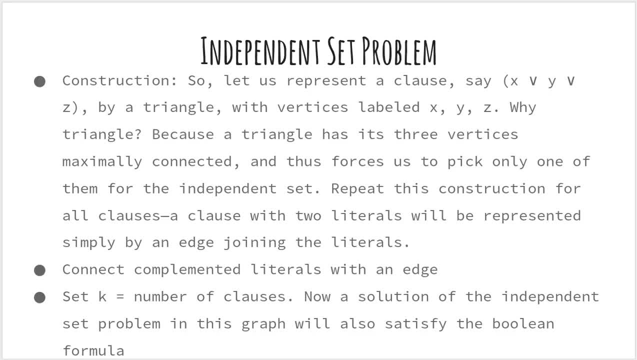 there will be an edge between 2 vertices of the independent set, which is not allowed. So once you repeat this construction for all clauses, a clause with 2 literals will simply be represented by an edge joining the literals, And since we have connected the complemented literals with the edge, 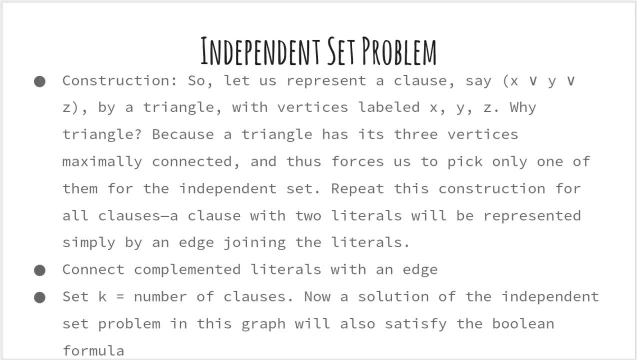 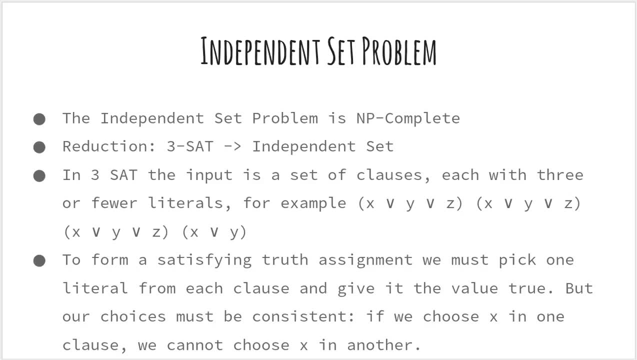 if we set k equal to the number of clauses, a solution of the independent set problem in this graph will also satisfy the Boolean formula. Now, this is plain to see because each clause we need to pick at least one vertex, because now we have said that we want a k-sized independent set. 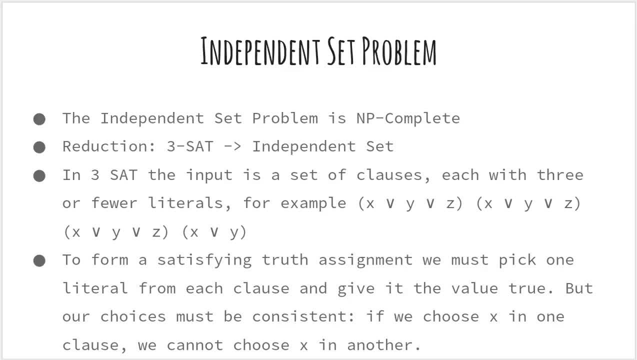 and a k-sized independent set will lead to a consistent solution. because, since we have said that there is an edge between every literal and its complement, we cannot possibly pick a literal and its complement to be a part of the independent set. Why? Because if we picked a literal and its complement to be a part of the independent set, 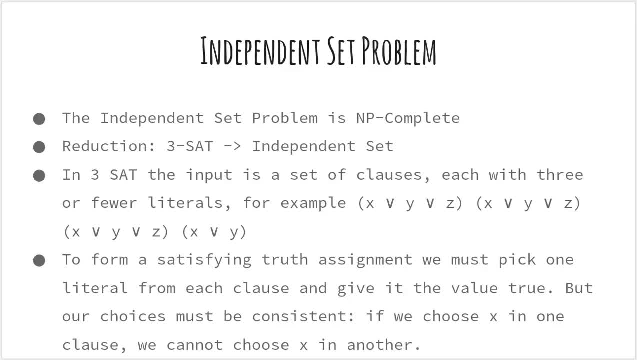 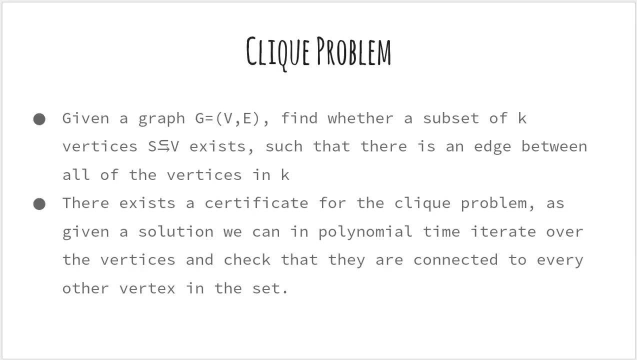 there would be an edge in our independent set which is not allowed So to form a satisfying truth assignment. we just pick one literal from each clause and give it the value true and we have consistent choices. So in this way we have shown that the 3-sat problem reduces to the independent set problem. 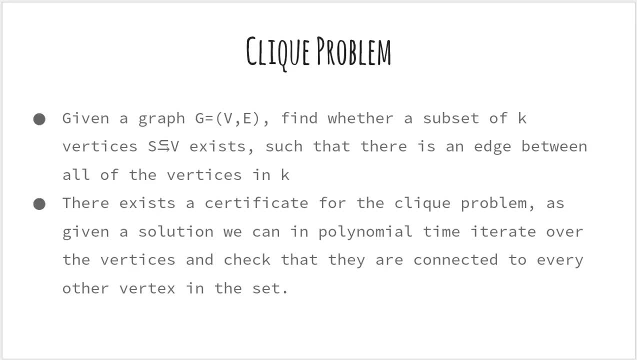 and that the independent set problem is NP-complete. Now we look at the clique problem, which asks that, given a graph G, can you find a subset of k vertices such that there is an edge between all of the vertices in the subset. So there easily exists a certificate for the clique problem. 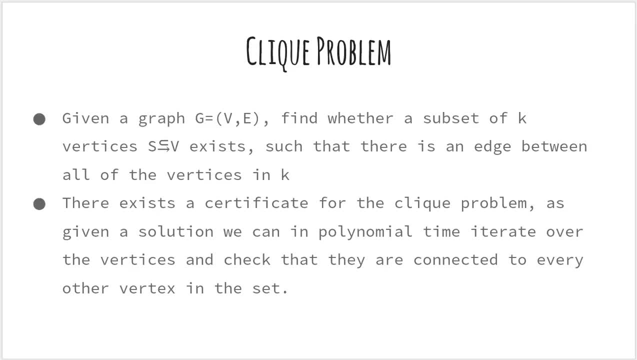 If someone gave you a k-sized subset, you can iterate over the vertices and check that each vertex is connected to every other vertex in the subset. So now we know that the clique problem is in NP. Now we have to show that the clique problem is NP-complete. 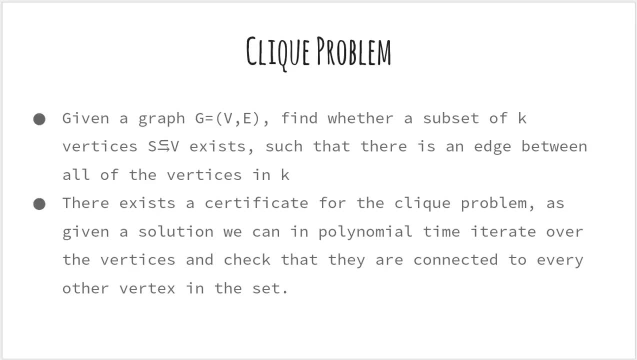 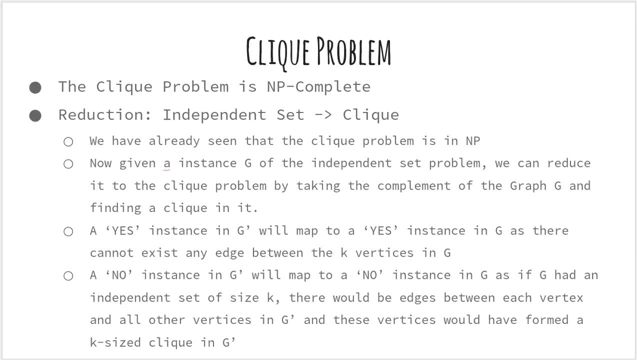 So the first step is choosing a problem to reduce to the clique problem. The NP-complete problem we will choose will be the independent set problem. So we have just seen that the independent set problem is NP-complete. So if you are given an instance G of the independent set problem, 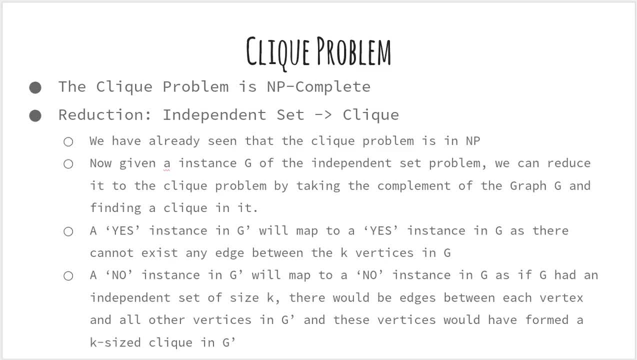 you can reduce it to the clique problem by taking the complement of the graph G and finding a clique in it. So the key idea over here is: you want to make sure that yes instances in your new graph G' map to yes instances in your graph G. 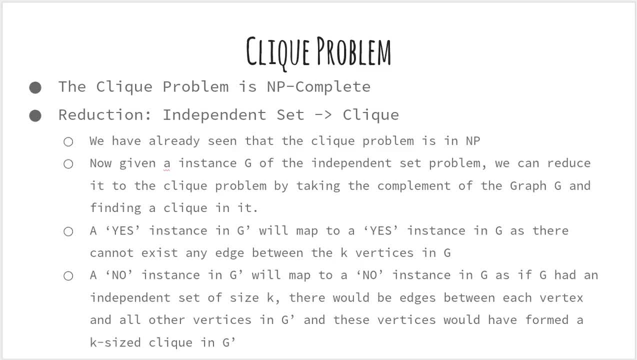 and no instances in G' map to no instances in G. So a yes instance in G' what does this mean? A yes instance in G' It means that a clique in G' maps to the presence of an independent set in G and the absence of a clique in G'. 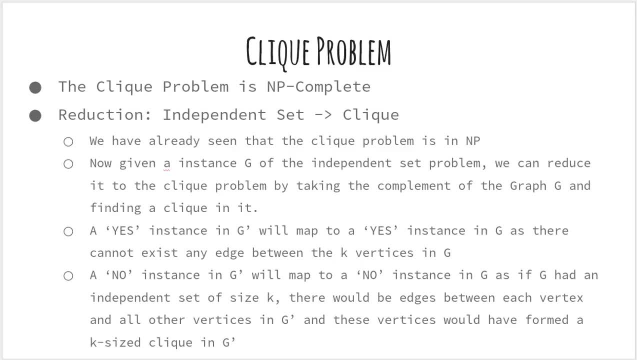 makes sure that there is no independent set of size k in G. So it's obvious that if you have a clique of size k in G' you will have an independent set of size k in G. Why? Because if you have a clique of size k in G'. 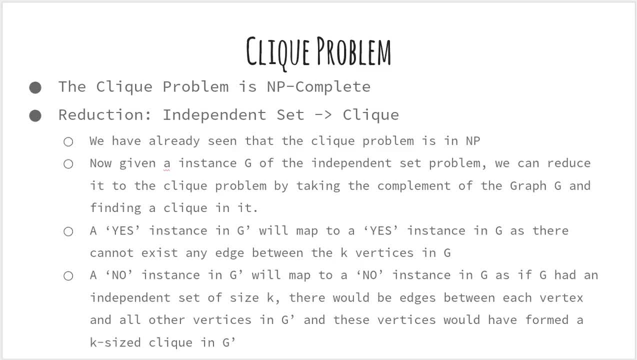 then each vertex is connected to every other vertex by edges. So if you take the complement of this graph which brings you back to the original graph G, none of these vertices are connected to any other vertex by edges, So they will form an independent set of size k in G. 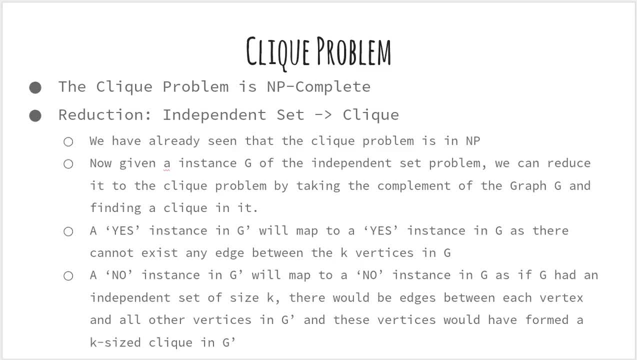 Similarly, supposing when you started in G, if you had an independent set of size k, there would be edges between each vertex and all other vertices in G' and these vertices would have formed a k size clique in G' So this proves that a no instance in G' will map to a no instance in G. 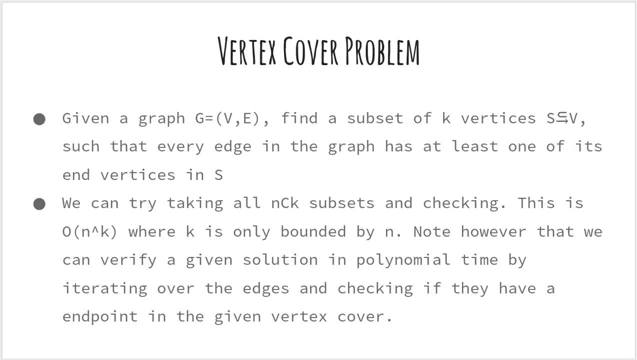 Alright, now we look at another problem, the vertex cover problem, which asks that, given a graph G, can you find a subset of k vertices such that every edge in the graph has at least one of its end vertices in this subset? One way of going about this is: 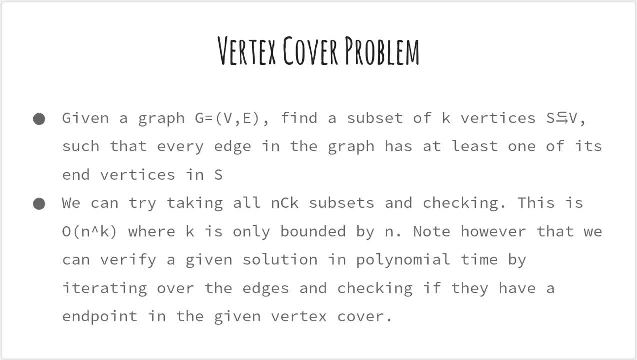 you can iterate over all n, choose k subsets of vertices in G and check whether they form a vertex cover. Finding whether these vertices form a vertex cover can be done in polynomial time. You simply iterate over every edge in the graph and check whether one of its endpoints 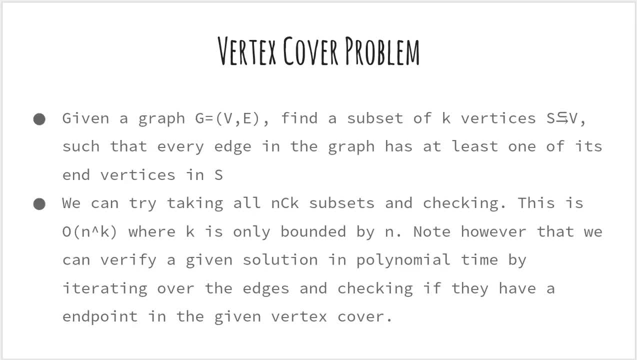 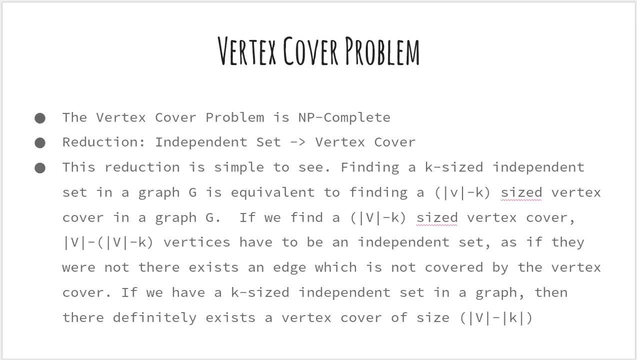 is within the subset you have chosen. So this is a certificate and it's clear that the vertex cover problem is in NP. But to show that the vertex cover problem is NP complete, we need to reduce a known NP complete problem to the vertex cover problem. 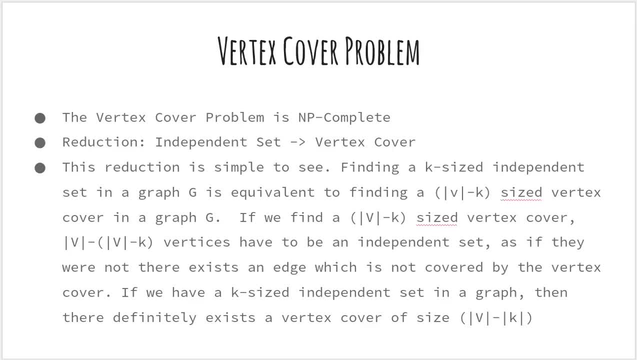 For this, we will choose the independent set. Now this iteration is simple to see: Finding a k sized independent set in a graph is equivalent to finding a v minus k sized vertex cover in a graph. Why is this the case? To do this, we will show that the yes instances map to yes instances. 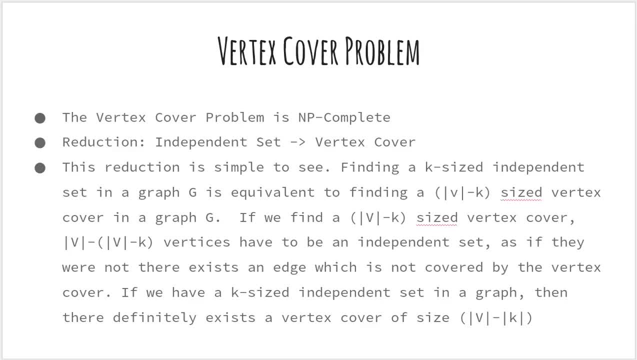 So if you could find a v minus k sized vertex cover, then it's clear that v minus v minus k, which evaluates to k, will have to be an independent set. Why not? Why? Because otherwise you have an edge between these vertices which is not covered by the vertex cover. 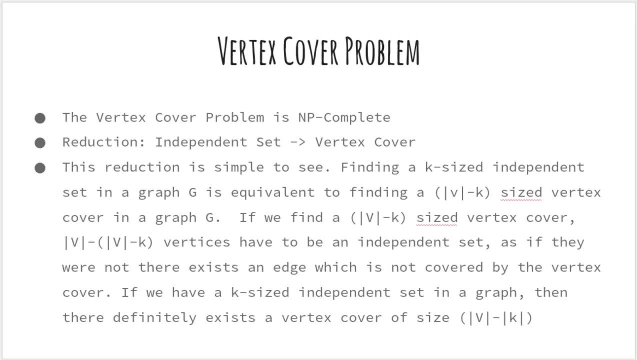 This is not allowed. Similarly, if you had a k sized independent set in a graph, then there definitely exists a vertex cover of size v minus k. Why? Because all the edges have to be amongst the remaining vertices, not amongst this k sized set. 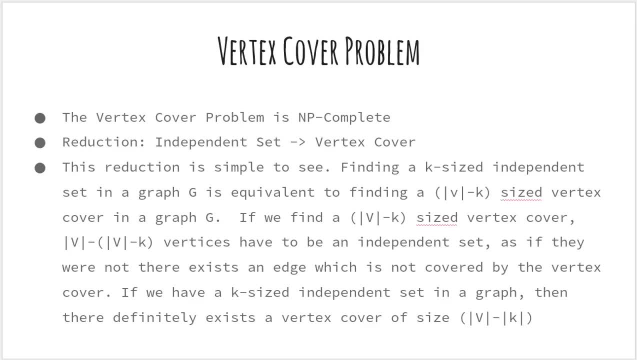 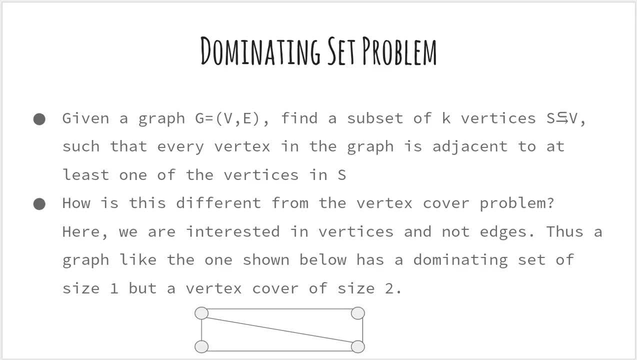 So thus we have shown that the vertex cover problem is NP complete by reducing independent set to vertex cover. Now we will look at the dominating set problem. The dominating set problem asks that if you are given a graph G, can you find a subset of k vertices? 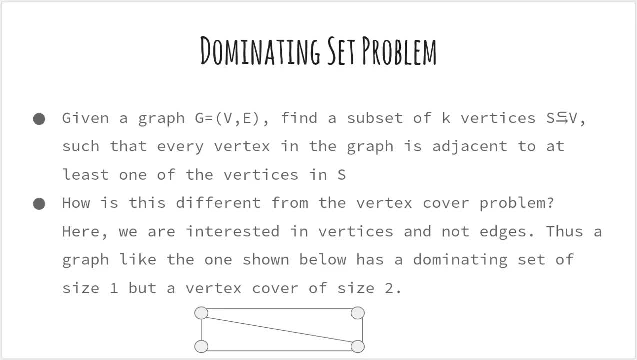 such that every vertex in the graph is adjacent to at least one of the vertices in this subset. Now these are different from the vertex cover problem, because here we are interested in dominating vertices, not covering edges. So a graph like the one shown, it's easy to see that. 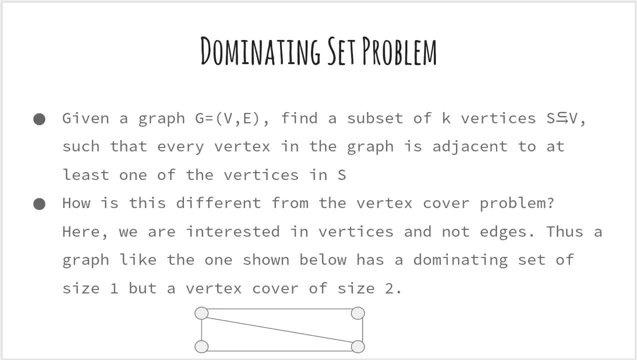 if you just pick one of the vertices, every other vertex is adjacent to that vertex. Thus it dominates every other vertex. So you can easily get a dominating set of size 1. But if you want to cover edges you need to pick at least two vertices. 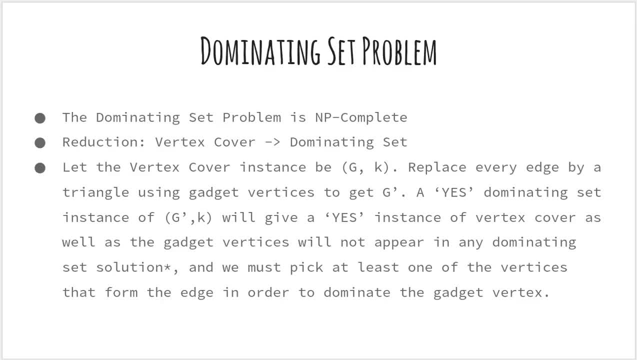 So you will have a vertex cover of size 2.. The dominating set problem is NP complete. To show this, we will reduce vertex cover to dominating set, Supposing you have a vertex cover, instance G. Now you replace every edge in G by a triangle using gadget vertices. 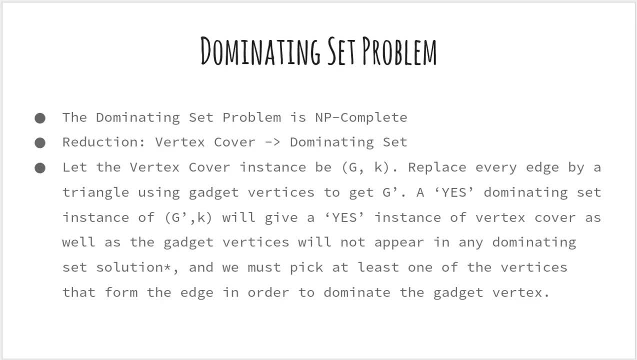 Gadget vertices are just artificial vertices we insert, So we make every edge in G a triangle, Now a yes instance of dominating set in G' which is a new graph constructed after replacing every edge in G with a triangle, will give a yes instance of vertex cover. 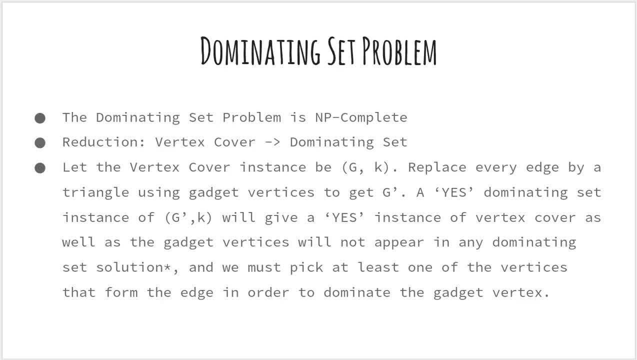 Why is this true? Because we won't pick any of the gadget vertices in our dominating set solution. Why? Because the gadget vertices can only dominate the two vertices at its end points. So we might as well pick one of those two vertices to be in our dominating set solution. 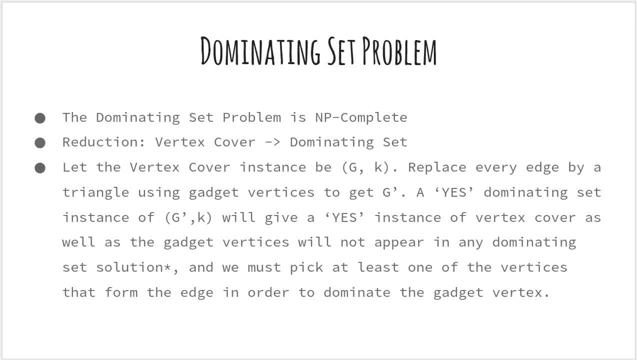 And we must pick at least one of these vertices that forms an edge, because they are the only vertices that can dominate the gadget vertices. In this way we end up covering all the edges. So this is essentially a reduction from the vertex cover problem to the dominating set problem. 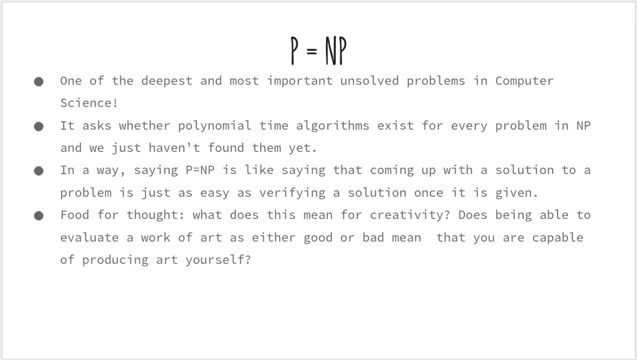 Alright, so now we have seen a set of NP-complete problems. A quick recap: We started off with 3SAT. We reduced 3SAT to independent set to show independent set is NP-complete. We reduced independent set to clique to show that clique is NP-complete. 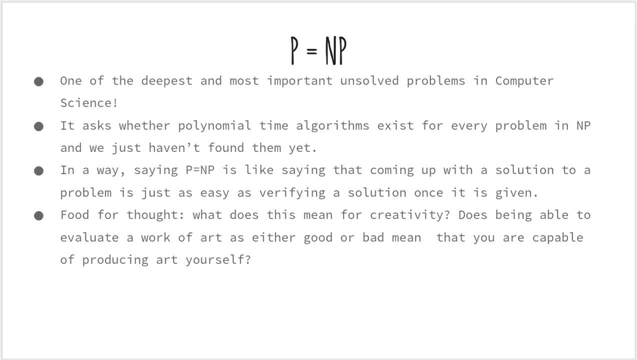 For vertex cover. we reduced independent set to vertex cover and showed that vertex cover is NP-complete. Then we reduced vertex cover to dominating set and showed that dominating set is NP-complete. Now we will talk about a very interesting question, which is: is P equal to NP? 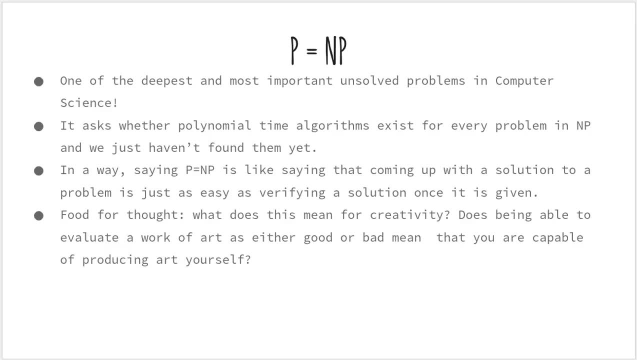 So we have seen that there are two complexity classes, P and NP, And what we are essentially wondering is whether we have polynomial time algorithms for all the problems that we know are in NP, and we just haven't found them yet. We know certainly that P is a subset of NP. 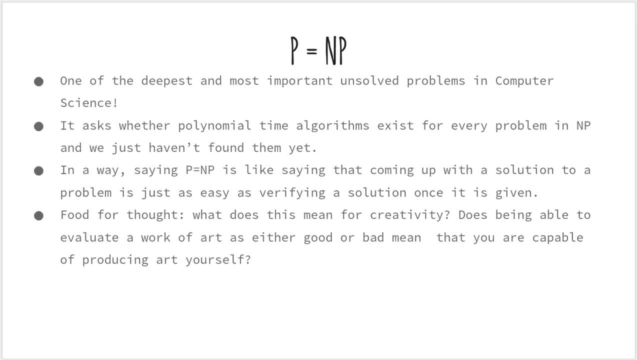 but the question we are asking here is: is it a perfect subset? So this is actually one of the deepest and most important unsolved problems in computer science. There is a prize of 1 million dollars by the Clare Mathematical Institute for the first correct solution to this problem. 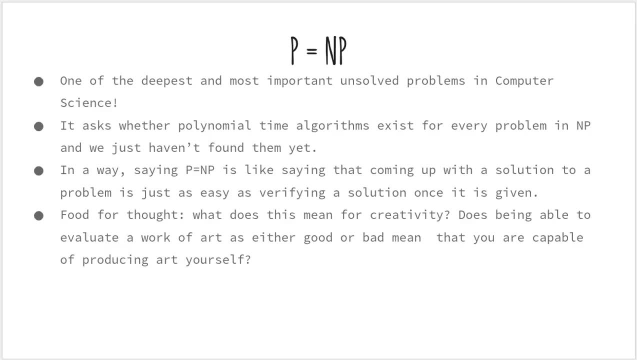 If we can get a proof either way about P equal to NP, it has a profound implication in a variety of fields, Because saying P equal to NP is kind of like saying that coming up with a solution to a problem is just as easy as verifying a solution once it is given. 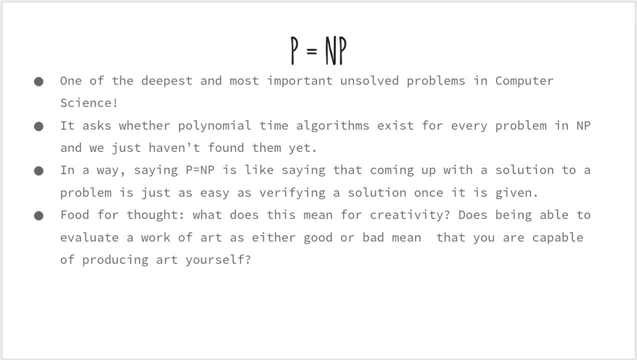 So you could think in layman's terms: what does this mean for creativity? Does being able to evaluate a work of art as either good or bad equivalent to being able to produce the work of art itself? Alright, thanks a lot for your time.